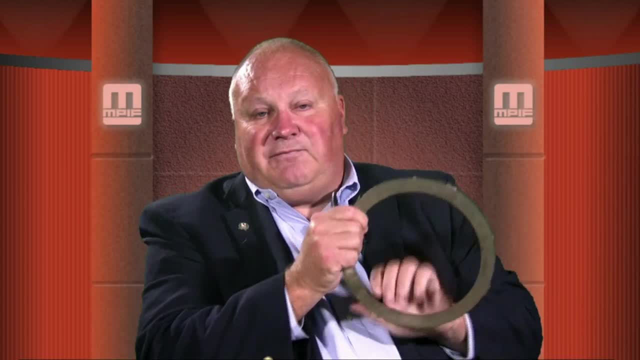 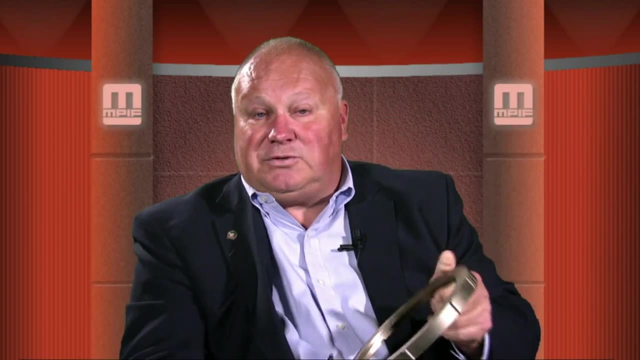 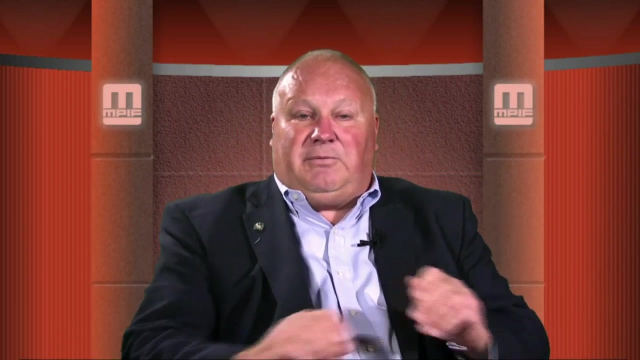 If the projected surface area of the part in the plan view is, say, 50 square inches and the powder that's being used requires 42 tons per square inch to achieve the desired density, a press with at least 2100 tons would be required. This is a little bit of a problem in that. 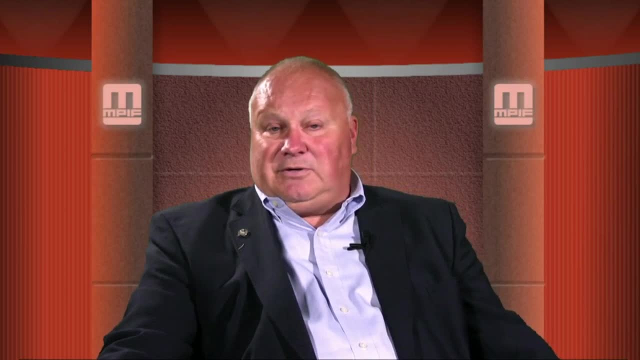 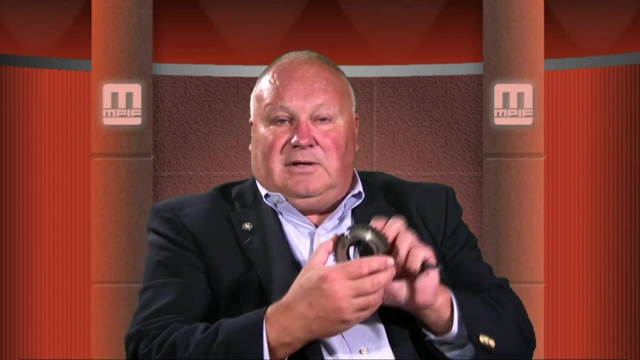 there are few, if any, presses in the 2100 ton range. So if we look at a PM part and we see the area in the plan view and let's take a look at a component this size, Let's say this is 20 tons per square inch. 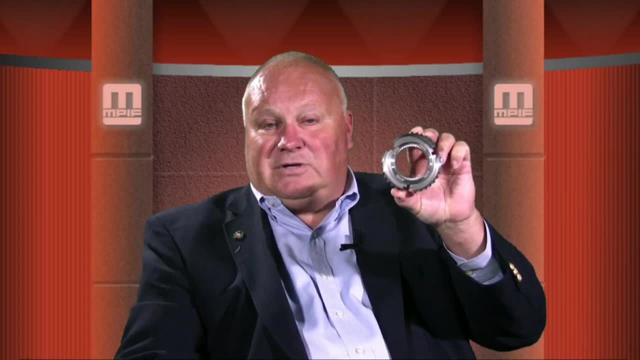 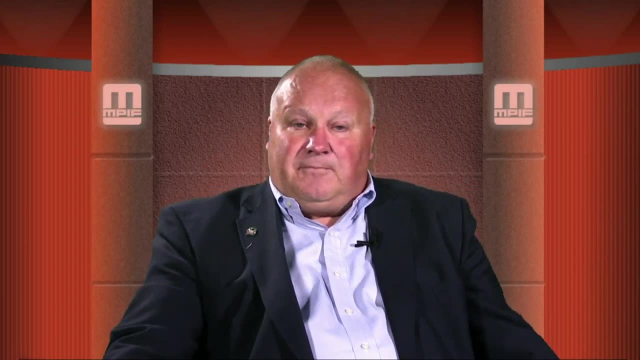 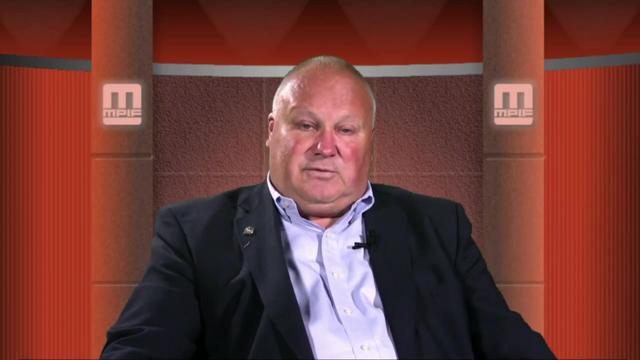 And again we use the same 42 tons per square inch powder compressibility to achieve density That would require around 840 tons. This is a feasible range for a number of PM parts makers And we start to get into a press size that the industry can manage. Another question: 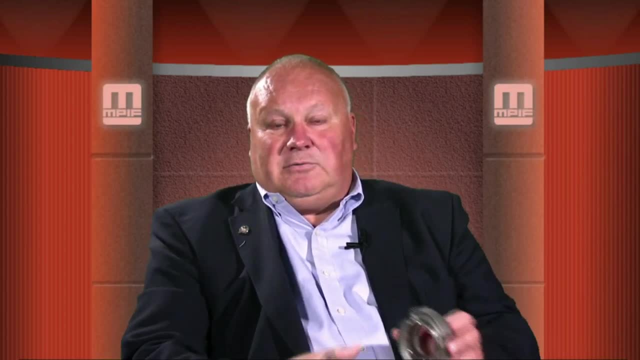 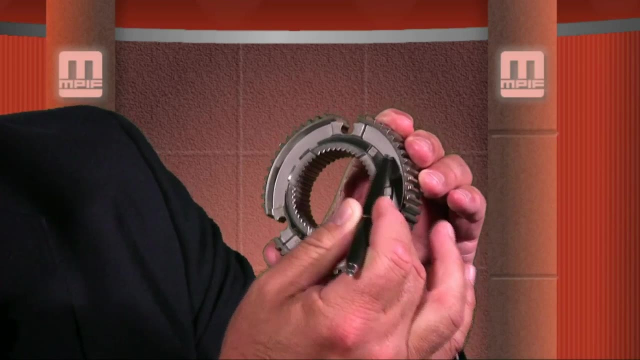 that we ask is how many part levels are required. When we look at a PM part, we count the levels. In this example you'll see 1,, 2,, 3, 4 levels. That would be the lower punch group Then. we have 1,, 2,, 3,, 4 upper levels. So you can see that we require 4 upper punches, 4 lower punch groups and a core rod and a die. So you're going to have to have a compound that. press with eight level part capability at least. Most multi-action presses have at least two lower and two upper level capabilities. There are also presses with three and four upper and lower levels. This is an example of a component. We look at a lower punch level, one lower punch level, two upper punch and a die. 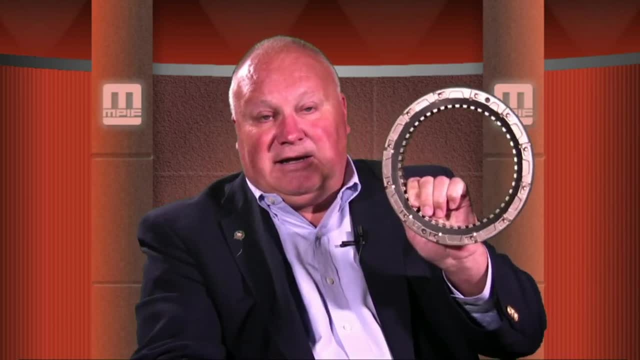 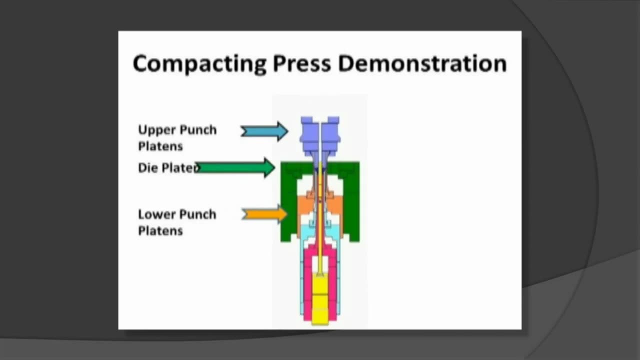 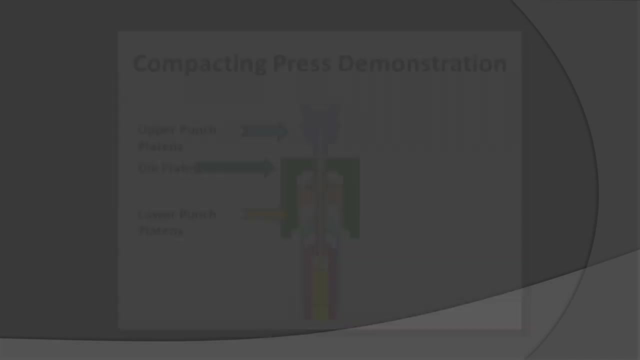 and a core rod to form the spline ID. This is an example of a compacting demonstration. You can see how the compacting press functions. Another question is: how tall is the part? We look at part thickness or part height this way, So 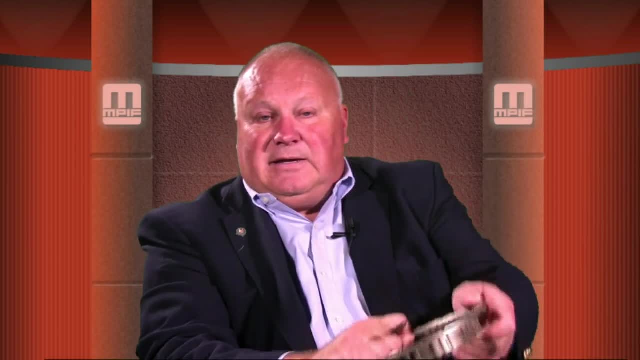 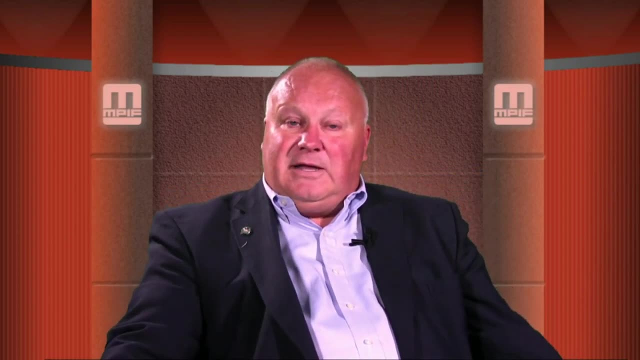 this would be the overall part height. Typically a part taller than two and a half to three inches would require presses with unique, or what we call deep fill capability. If a component is particularly tall, we can braze or join two parts together. The next picture is a great example of components that have 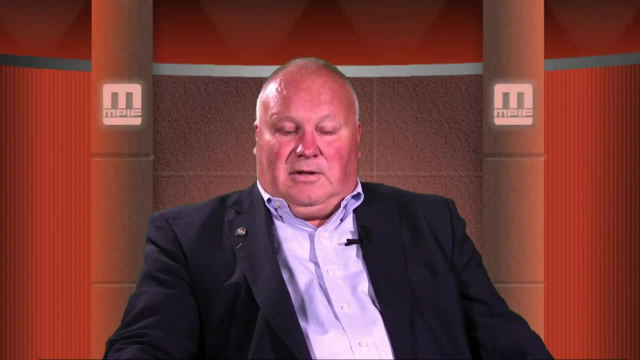 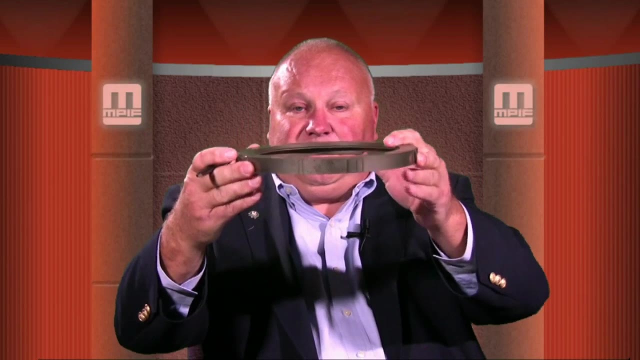 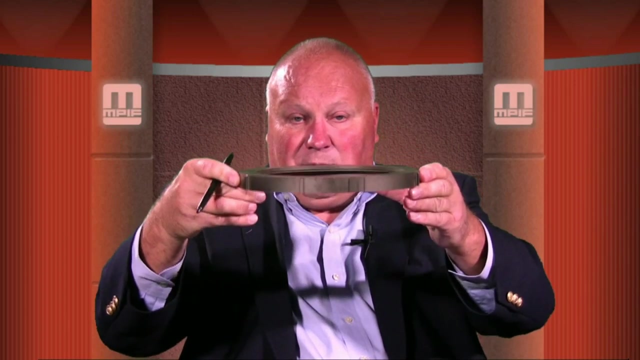 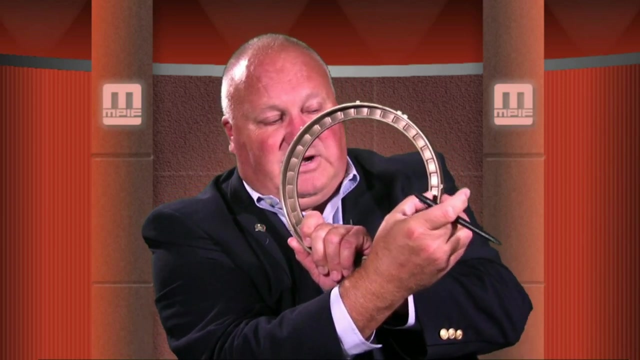 been used using the center brazing process. Another consideration is aspect ratio. When we look at a PM part, we look at this component and this would be the direction of pressing. This way, we see that we have a fairly low aspect ratio part. However, within that part, we see this low aspect ratio wall thickness. We 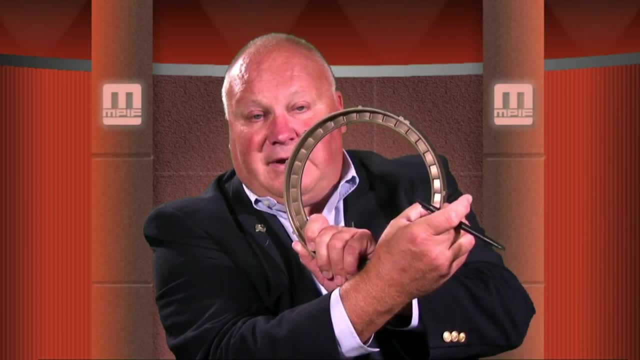 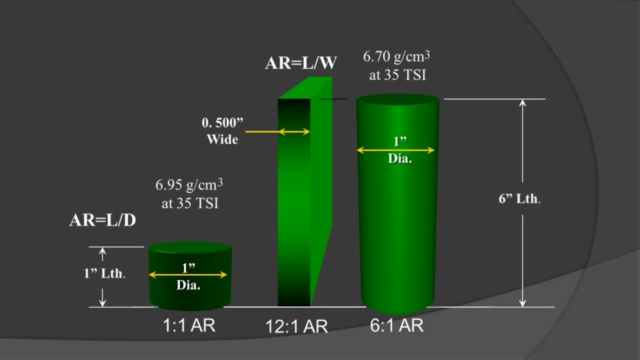 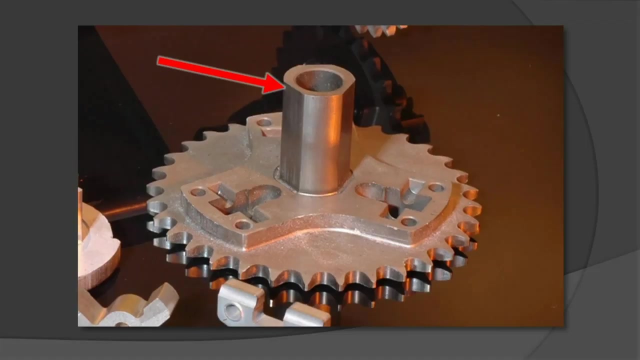 need to pay attention to that aspect ratio when considering PM part design. One-to-one is very good, A six-to-one is feasible and greater than 12-to-one can be very challenging. The next example: you'll see a picture of a PM component that has 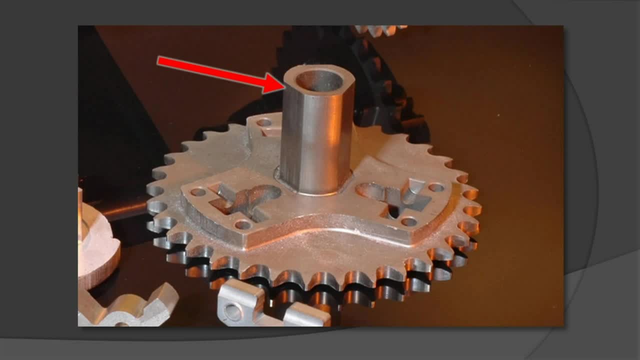 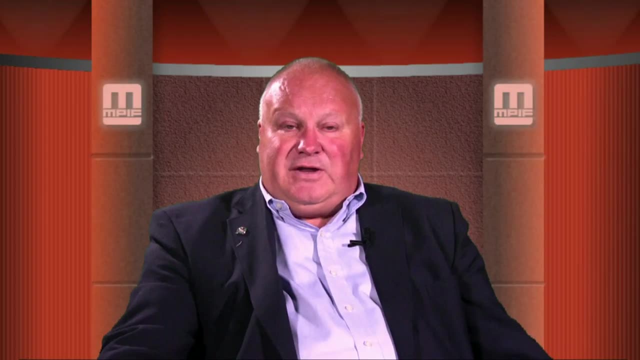 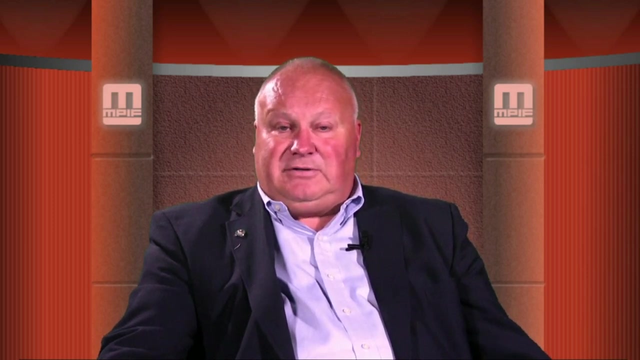 a 15-to-one aspect ratio in the flat section of the component in the wall. In some instances there's features that can't be pressed into the part. Grooves are a good example of features that typically are not pressed into the component. Here you see this large ring. 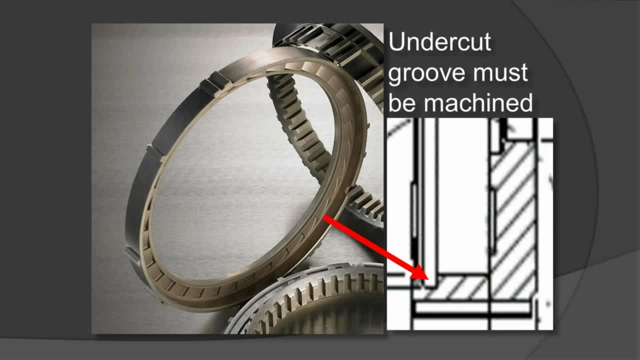 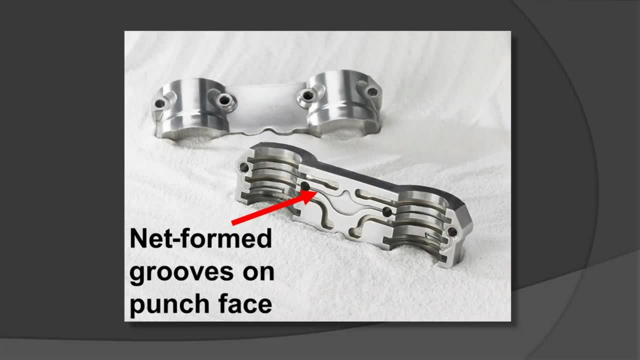 and we're machining a groove according to the drawing in the component because that part cannot be pressed. These are examples of net formed grooves on a punch face and these can be compacted into the PM part. The next question is: what are the properties and the functional requirements of the component, Since PM can provide excellent properties in the right application. material selection and part processing are very important. The material standard, MPIF standard 35, provides a comprehensive structure for specifying a variety of material and process options. When looking at material options, there are a number of questions to consider. The material composition can. 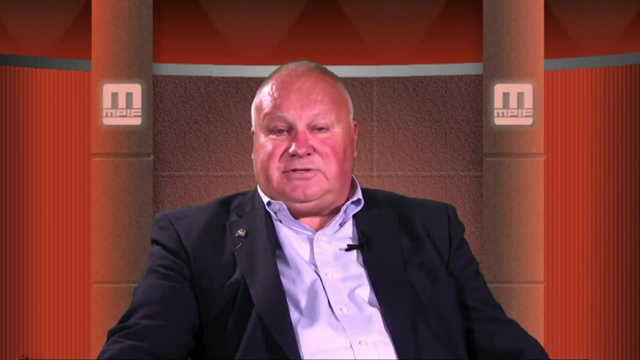 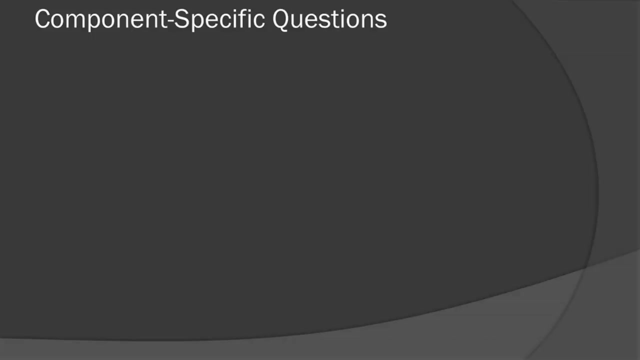 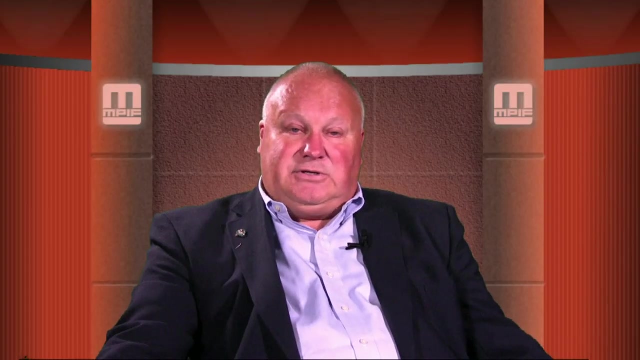 affect dimensional stability. response to secondary processing, such as heat treatment and machining, Strength requirements, wear and secondary operations also influence material selection. Some component specific questions, such as: will the part operate under a fluid pressure? Must it be leak tight? Parts that are used in pneumatic. 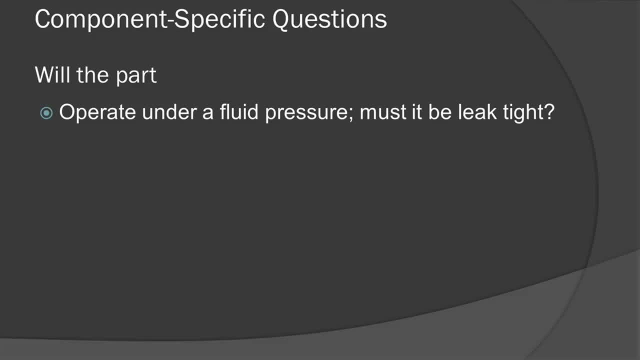 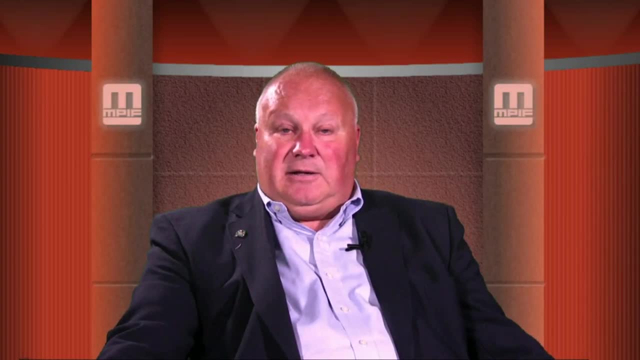 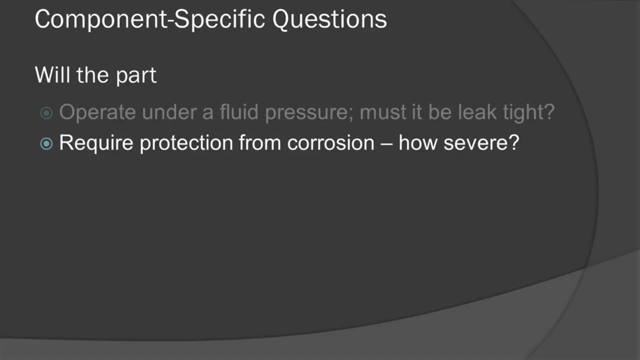 and hydraulic applications cannot leak. Must the part require protection from corrosion? If so, how severe? Will it be used in a marine environment, or do we need simple ambient corrosion to protect it from room conditions? Will the part require machining? If so, which surfaces and what tolerances are required? Will a 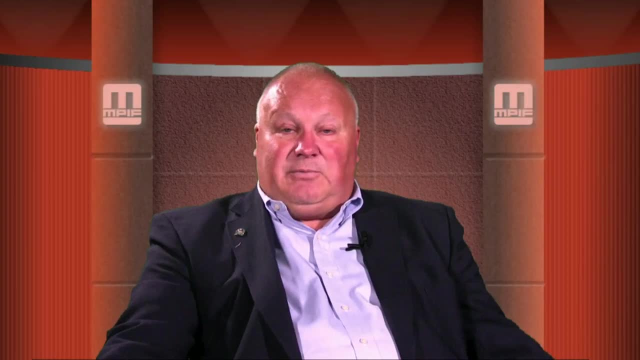 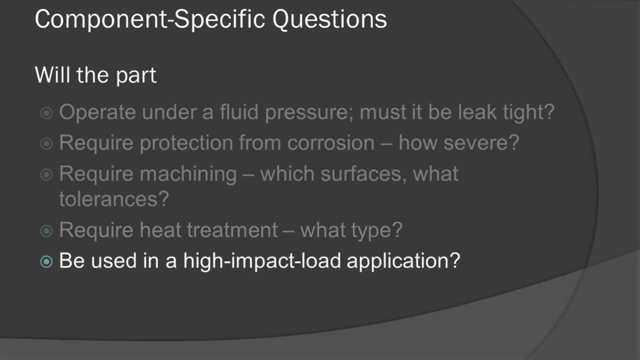 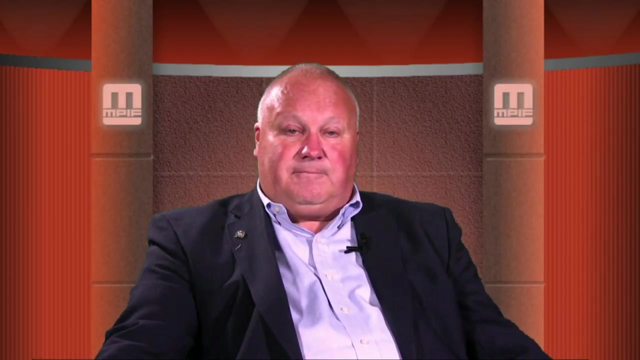 component require heat treatment? If so, what type? Can we use a center hardened material or do we need to use a quench and temper material? Is the component used in a high impact application where high impact loads must be endured? Will it be used in? 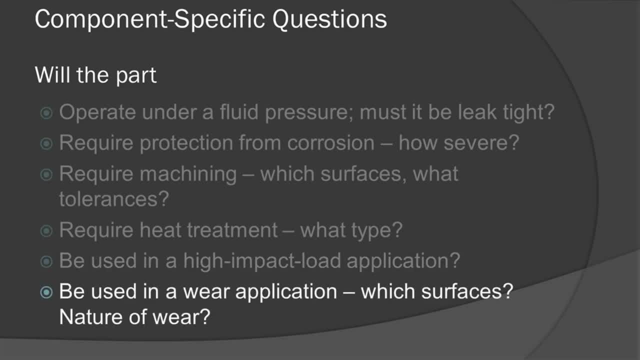 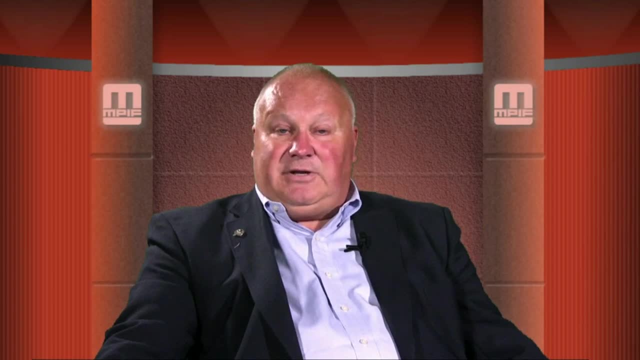 a wear application? If so, what surfaces and what is the nature of that wear? Is it a high contact stress application, such as you might see in a heavily loaded gear? Will the part be used in a magnetic application? Is it a soft magnetic application or a hard? 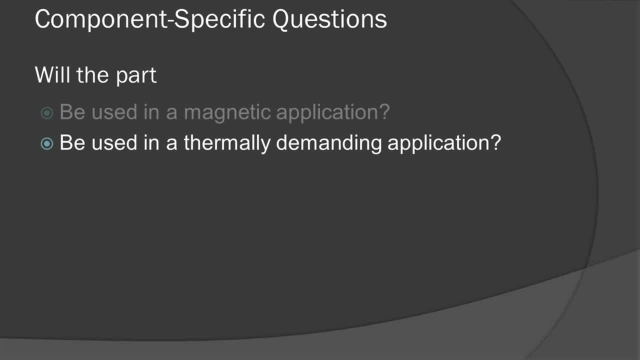 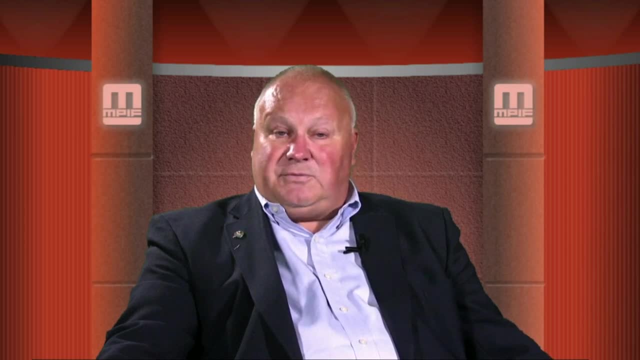 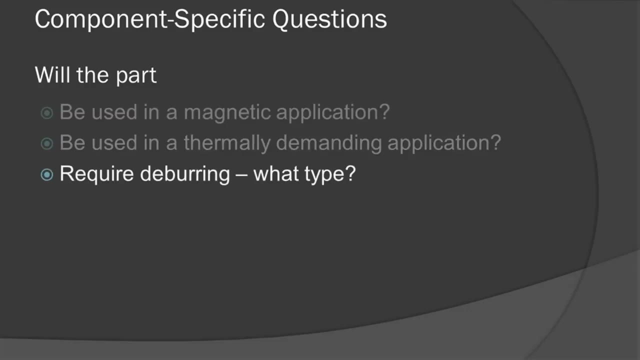 magnetic application. Will it be used in a thermally demanding application? Will it such as an exhaust system, Exhaust system? components need very good corrosion resistance. Strength is also a consideration at elevated temperatures. Will a component require deburring? If so, what type of deburring is appropriate? Can it be deburred in the green state prior to? 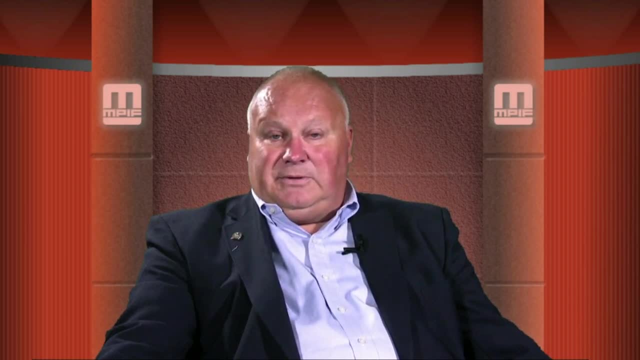 sintering or must it be vibratory, finished or tumbled? What kind of corner, brakes and radii are required? What other deburring requirements might be important? Will the component be welded? Powder metal parts are porous Parts that are filled with oils and fluids don't readily weld. 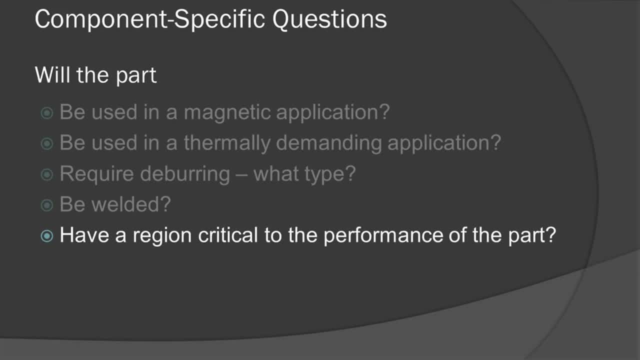 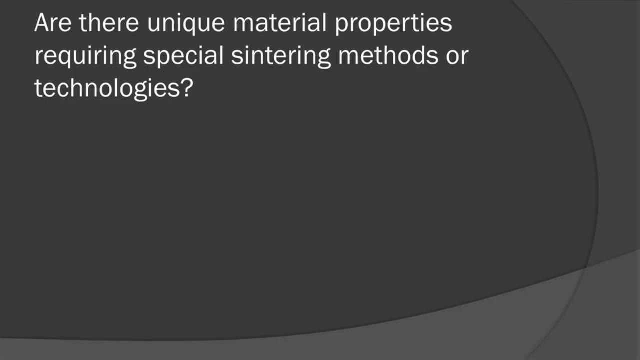 Is there a region of the part that's critical to the performance? And again, one of the questions we need to ask is packaging. Will unique packaging requirements apply? Must they be returnable packaging or can we bulk pack in containers? Are there unique material properties requiring special sintering methods or technologies? 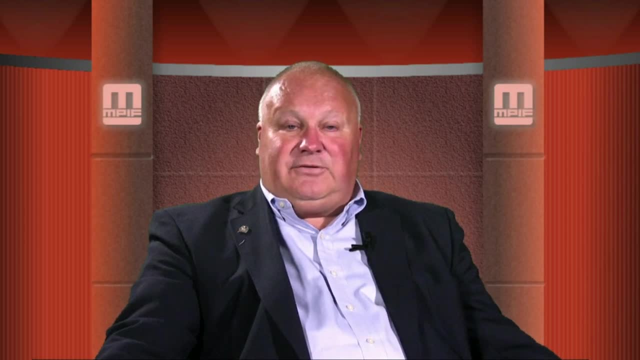 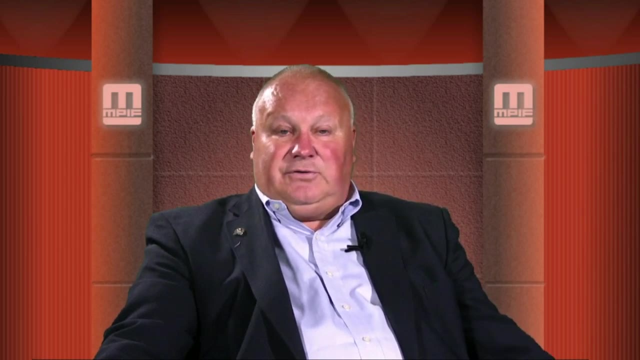 Plain iron materials and iron carbon steel alloys are readily sintered at conventional temperatures in the 2050 to 2100 degree F range and atmospheres using nitrogen and hydrogen or endothermic gas. Highly alloyed materials, such as stainless steel tool steels, are best sintered at elevated 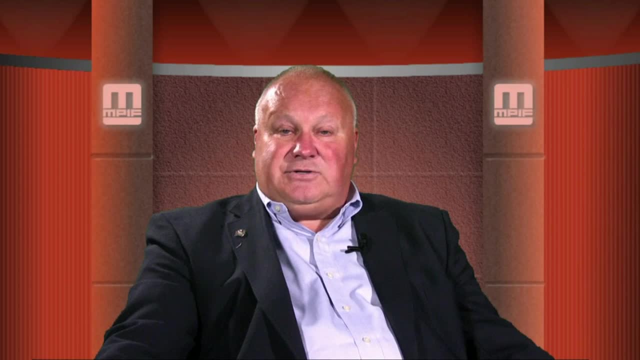 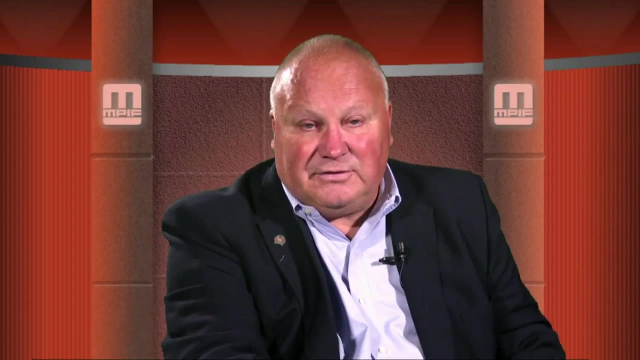 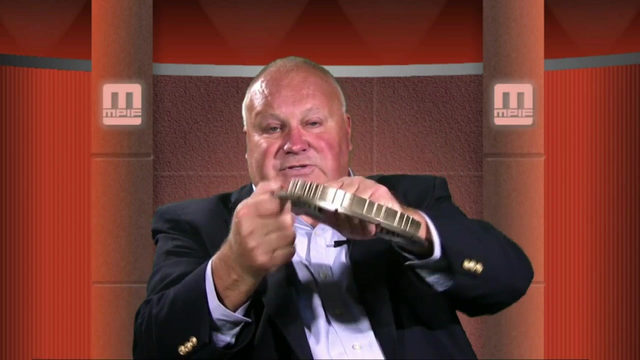 temperatures in the 2350 degree F range or greater, and pure hydrogen or vacuum atmospheres, Parts requiring low flatness. we look at a part like this, this direction. we may choose to center on special fixtures to keep this face flat and these surfaces very parallel.